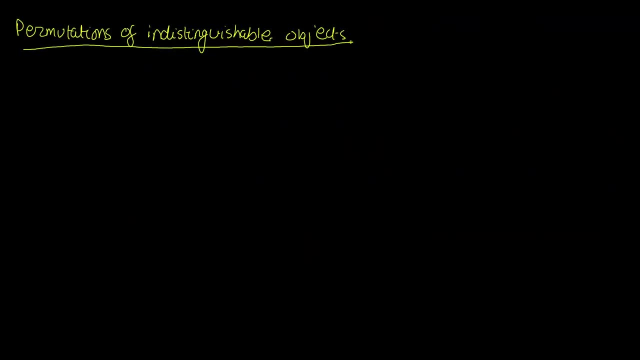 of indistinguishable objects. So the first thing that we want to do is to clear out any confusion regarding indistinguishable objects versus repeated objects. We have already had a look at repeated objects in yesterday's video, under permutations and combinations with repetition, And the main idea in repeated objects is that each object could be chosen more than once. 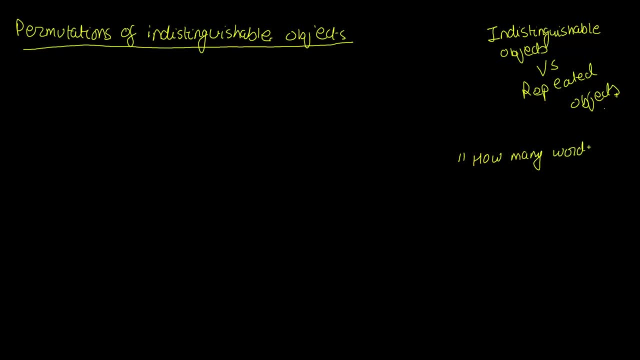 For example, we looked into a problem like how many words of four letters are possible And for this question we argued that there would be 26 different letters to choose from And we have four positions where to put those letters. And in the task of forming words from letters, repetition is allowed. So there would be 26. 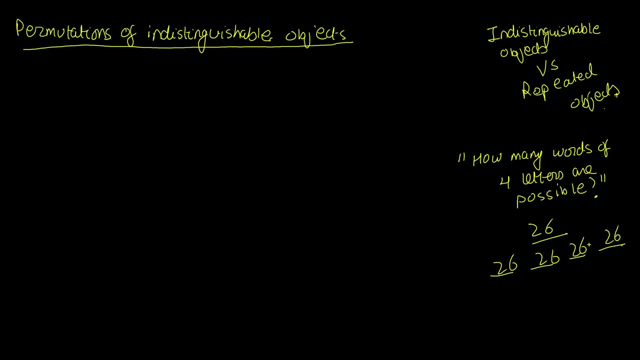 choices for each of these possibilities And we concluded that the number of ways for this would be 26, raised to the power of four. So when we're talking about repeated objects, we have a fixed number of objects and we can choose any of them more than once. 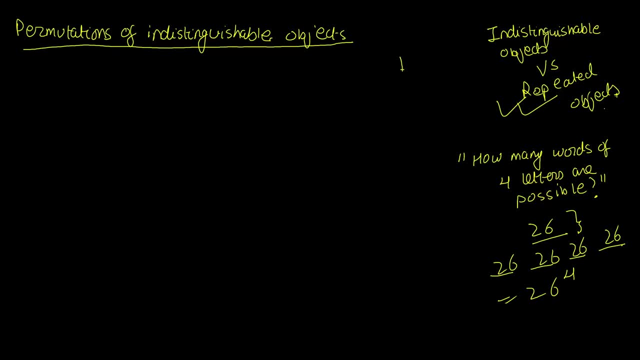 But now, if we consider this question, in how many ways can the letters of the word dad be arranged? Let me write the possible arrangements to show what I mean. I could either write an arrangement called, let's say, DDA. it could be a, followed by two Ds. 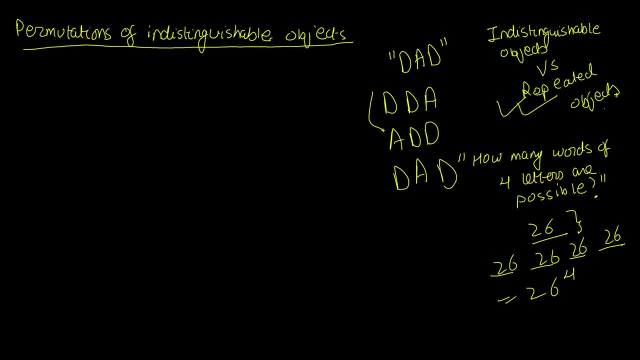 or it could be an A sandwiched between the Ds. These three are the three possibilities of permitting the word dad, And I want you to be able to see the difference between these two problems. Here, the words that are given to us are fixed. we have to work with exactly two. 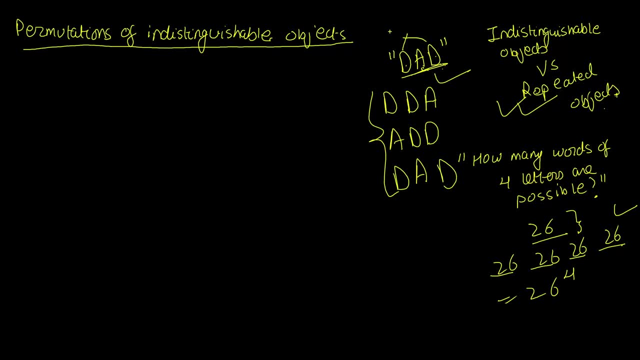 Ds and exactly one A. So in this case we say that this D and this D are indistinguishable. So when we're talking about repeated objects, we know what the different categories are and we are allowed to choose zero from each category or any number of items that we want. 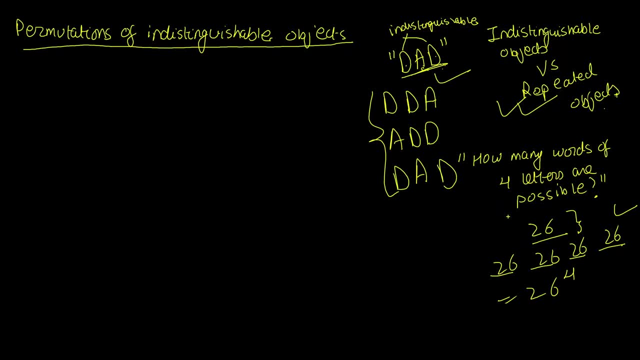 from each category. When I'm making four letter words, I have 26 different categories And that comes from the 26 different letters available to me. But when I'm picking each of my letters to form this word, not all of the 26 letters will be in these four positions. 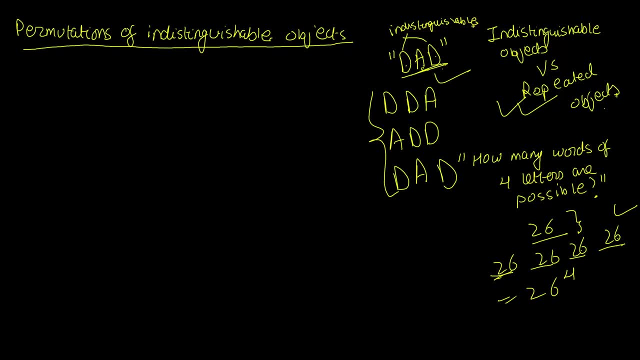 But when we talk about indistinguishable objects, the objects by themselves are fixed. we know what goes into the selection. it is just the fact that not all objects are distinguishable. So this D is the same as this D. So I hope you can see the difference between. 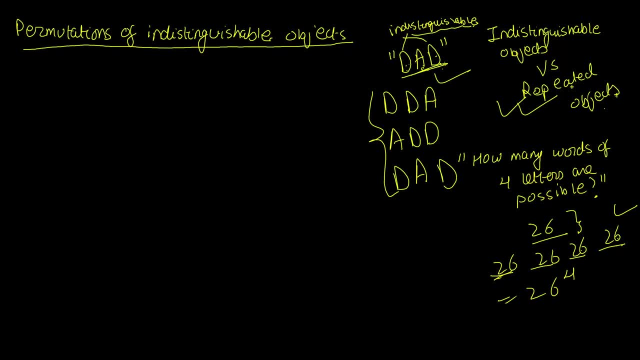 things being indistinguishable and things being repeated. So let us look into this particular problem in a little bit more detail. So, like we talked about, I want to take a word, like dad, in which all the objects are not distinguishable and count the number of permutations of arrangement of those objects. 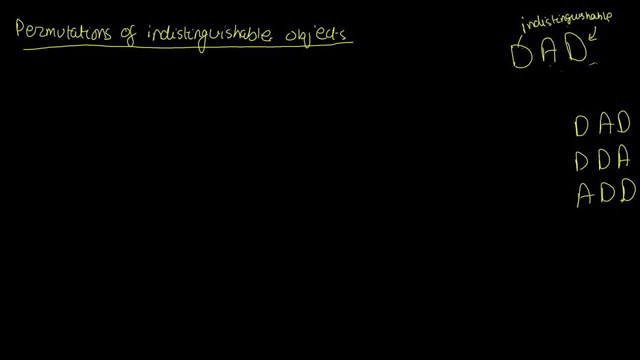 So we already saw for this example there are three different permutations, But how do we know that it is three? so we can approach a problem like this in two ways, And both of them lead to the same solution. The first approach borrows the result from earlier: the number of permutations. 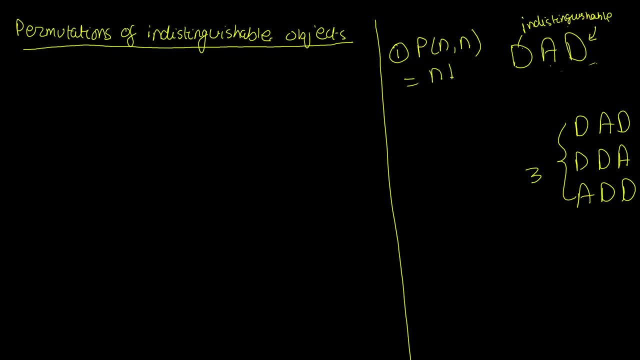 of n things taken all at a time is just equal to n factorial. But we know this only works if the items are distinct or distinguishable. So we start by assuming that they are. if these three letters were distinguishable, the number of permutations would just be equal to three. 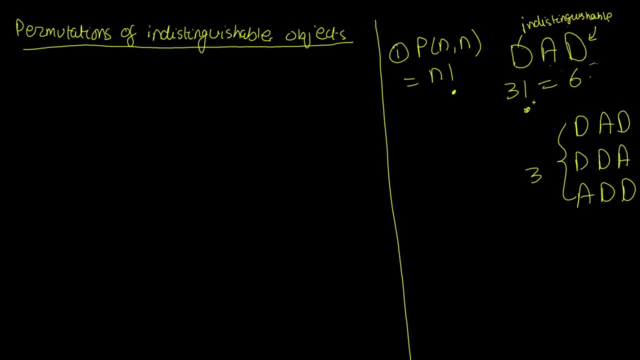 factorial and that would be equal to six. But I know that the final number of permutations will be lower than six because some items are indistinguishable And changing the permutations within those items wouldn't result into a different permutation. Therefore my answer. 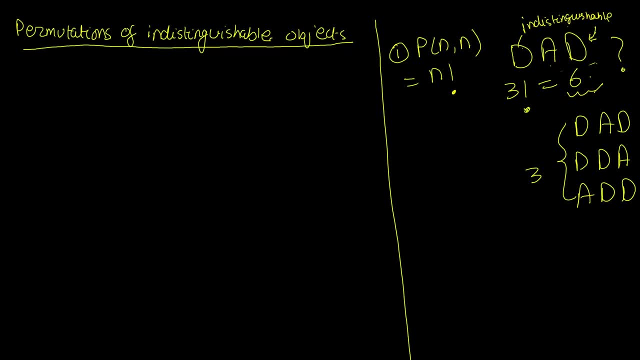 is definitely going to be less than six, But by what factor? So if I look at my word, I see exactly two D's, And the two D's can be placed in these two positions in two factorial ways, assuming they were distinct. Therefore, the total number of permutations reduces by a factor of two. 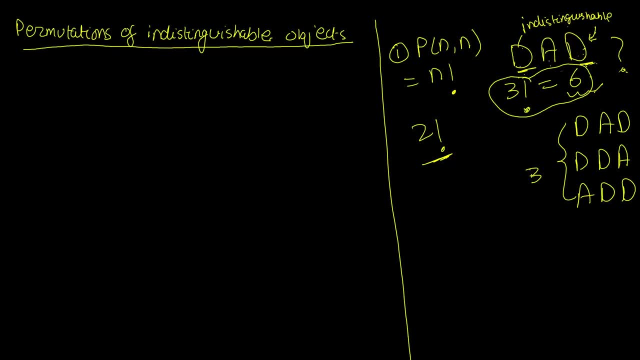 factorial, And so that is one way to reach the answer. I begin by saying: if all letters were different, there would be three factorial ways, But within these three factorial ways there are two distinguishable pairs of D, and the two factorial arrangements within D will result. 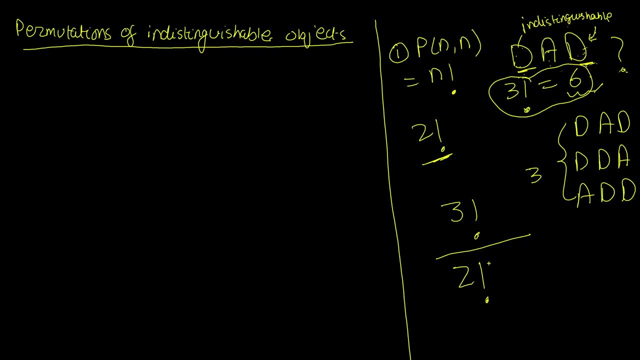 into the same permutation. So my answer would just be three factorial divided by two factorial. In this case it would just be equal to three. But I can also view this problem in this way: For three different letters, I consider there are three different. 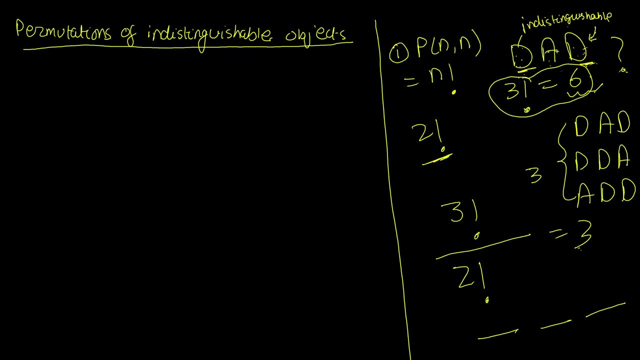 positions And my job is to put two D's. you know I have a total of two D's and one A, So two D's and one A should be put into these three positions. So in order to put my two D's, I'll choose any two random positions out of three. 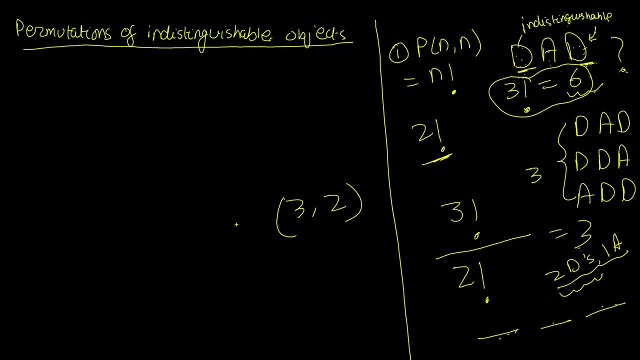 So out of three, I want to choose two positions, But will this be a permutation or a combination? I hope you can see that the order of my choice does not matter and I should be taking a combination. That is because when I select any two random positions in order to place D 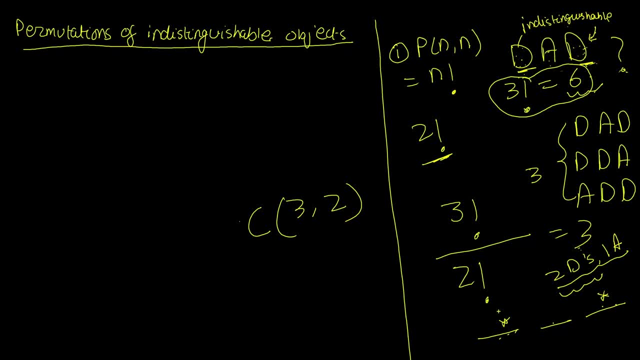 the order in which I select them does not matter. If I select this one first and this one second, I'm going to get a D here and a D here. But if I happen to select this one first and this one second, that still creates a D here and a D here. So since this D is indistinguishable, 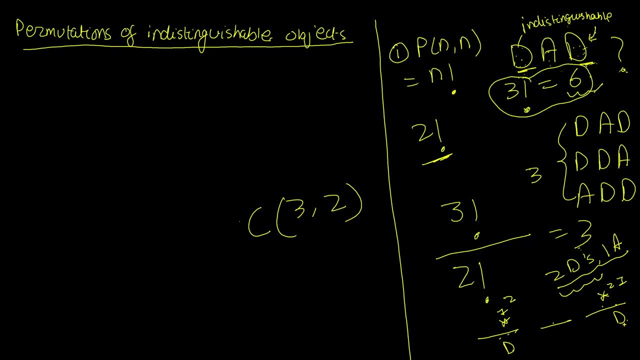 the order in which I select to place them does not matter. So I'm selecting a combination of two things from a total of three positions, And this gives me a total number of ways that I could place D in my three positions. Now on the remaining one. 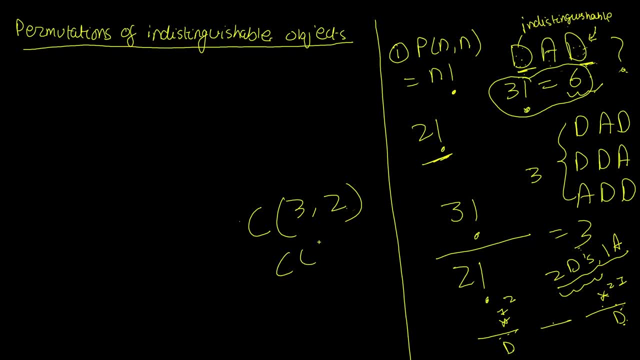 position. I just want to place the A, and that will be equivalent to C11.. There will just be one way to do that. Therefore, the total number of ways of permuting the world is going to be the product of these two possibilities And if I apply the formula for combination, I know that C3,2 is just 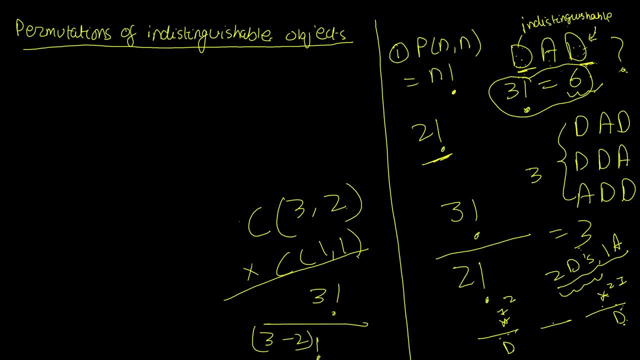 equal to three factorial by three minus two factorial times two factorial, And I hope it's easy to see why this is the same as this expression. So I'm going to place D in my three positions. This part will just be one factorial and three factorial by two. factorial is the number that I'm 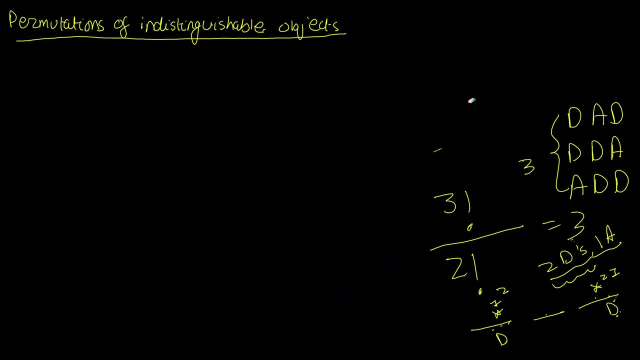 looking for. So let us do a quick and actual problem on this category, And we'll make sense of this even more. So exactly the same problem as we discussed earlier, but I'll choose a longer word And we'll do this formally this time. In how many ways can the letters of the word? 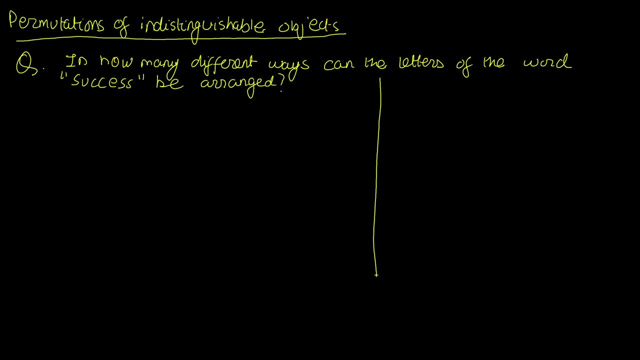 success be arranged. Okay, so two ways to solve this problem, as we saw with the problem with the word dad. So I could start by considering that there are seven different positions for this word. with seven letters, I see that I need to place three of S, one of U, two of C and one of E. So out of my seven, 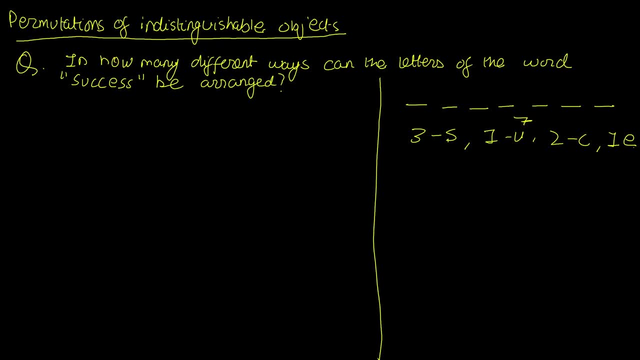 different positions. I'll select any random three for my S And from my earlier discussion I know I should be taking a combination, So I'll take C7,3.. Now the next biggest occurrence is of C. there are two of C's And after placing these three occurrences of S, I will have seven minus. 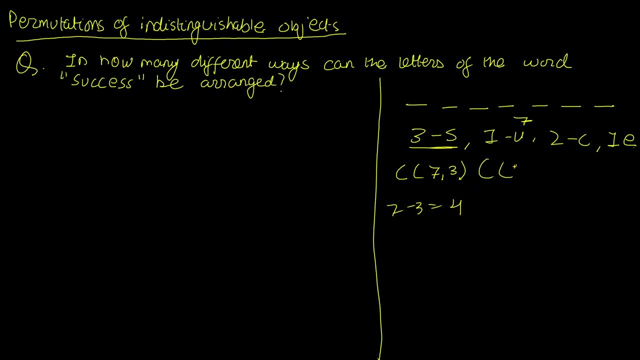 three is equal to four spots remaining. So out of the remaining four spots, I'll choose two for C. So after this, five out of seven spots are gone. So out of the remaining two, I'll select one for U, and the remaining one should be selected for the E. 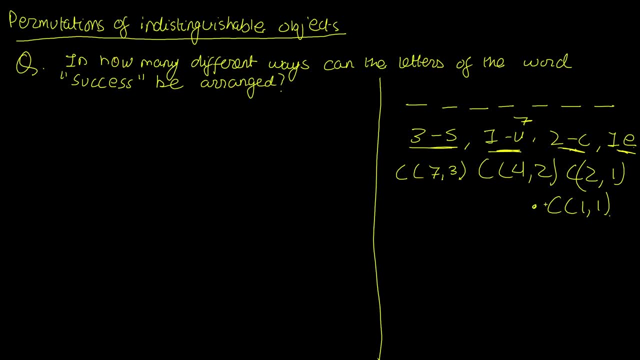 Now, before we evaluate this, one quick remark. I'm not necessarily required to consider these letters in descending order. When I had seven different positions, to start with, I assigned three of that to S because three was the biggest frequency. But that was just a convention. I could have started with anything that I wanted. So if I write this expression, 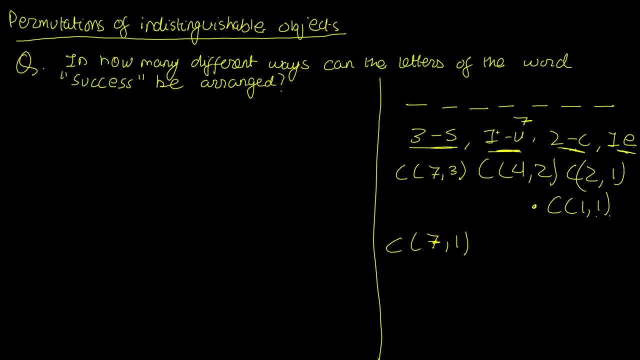 C7 comma one, suggesting that out of seven spots I'm assigning one for U, and then I could maybe say C6 comma one, meaning that for the remaining six spots, after placing U, I want to assign one for E. you know so, out of the six, one for E, And now five spots remain, let's assign two for C. 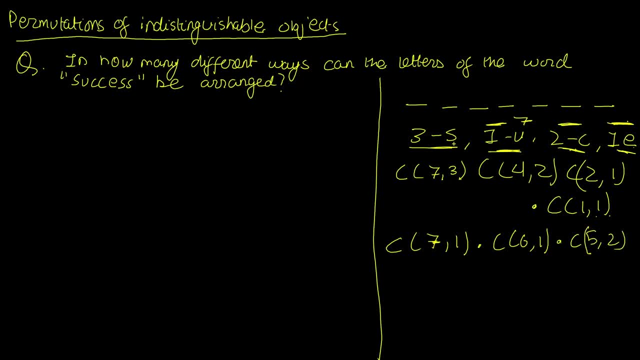 So I'll just say C5,2.. And now we'll assign S last. we have three spots remaining and we'll assign S in those three spots. So it will just be C3 comma three. So if you were to do the same thing, you will get exactly the same number. it's going to be equal to 420. 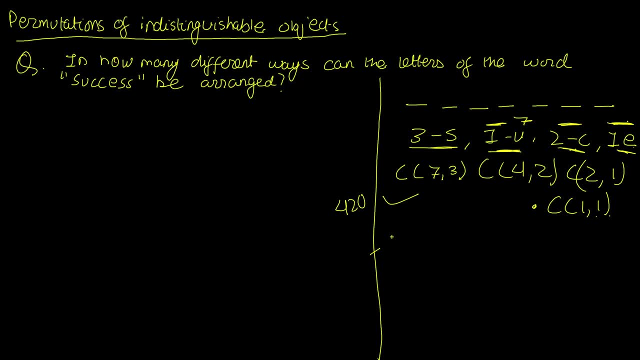 So let me expand the first one. So the first combination is going to give seven factorial by three factorial times four factorial. The second combination- you can apply the formula- will give four factorial by two factorial times two factorial. The third combination, quite easy. 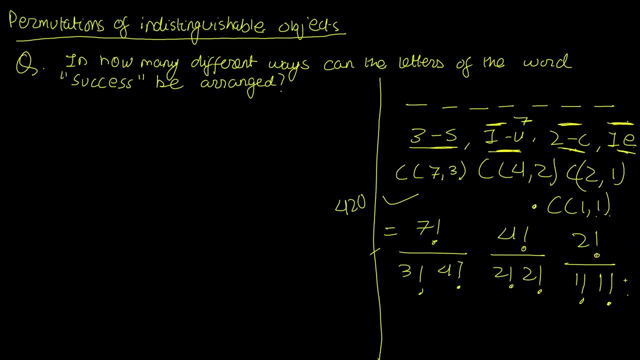 And the fourth combination will just be one. I'm not mentioning it here, But the idea that I want to show you is that in this fraction there is cancellation in a chain. So this four factorial is cancelled with this one, these two factorial cancels against this one. So if I show you, 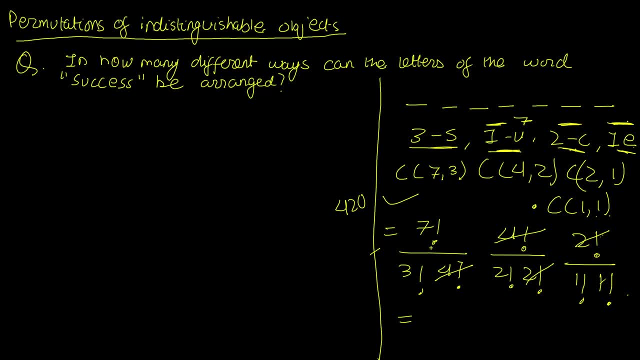 ultimately, what remains, only the very first factorial will remain, And this seven corresponds to the total number of words in here or the total number of positions that I assumed in here. So my numerator is going to be seven factorial. And if you look at what remains in the denominator, 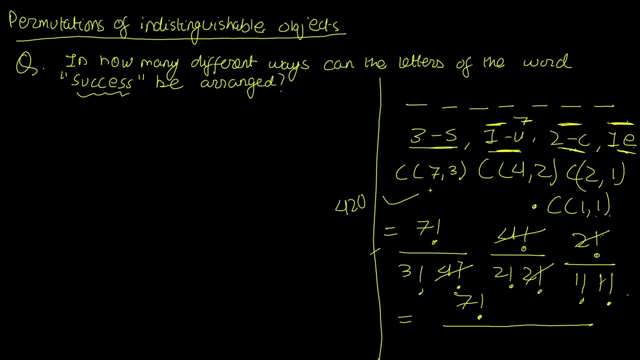 you'll be able to observe one factorial term for each indistinguishable group. So if I have three occurrences of s, I have a three factorial in my denominator. Since there are two occurrences of the c, I also have two factorial in my denominator. 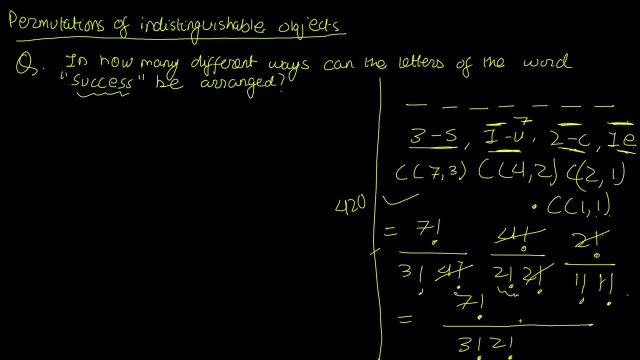 that comes from this term. Similarly, for the one e, I'll have one factorial in my denominator And if you remember, we did not mention one more term here. there was one more term here and that will give another one factorial in the denominator. So I think this is the formula that you are familiar. 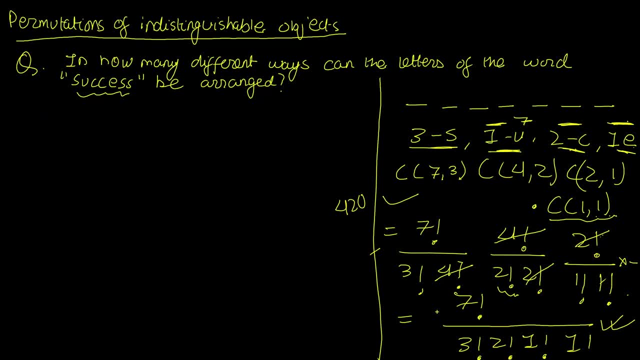 with, And if you're answering this question in your exam, you are allowed to use this formula directly. It is generalized And widely known, So your answering argument could look something like this: The permutations of the seven letters of the word success corresponds to the permutation of seven. 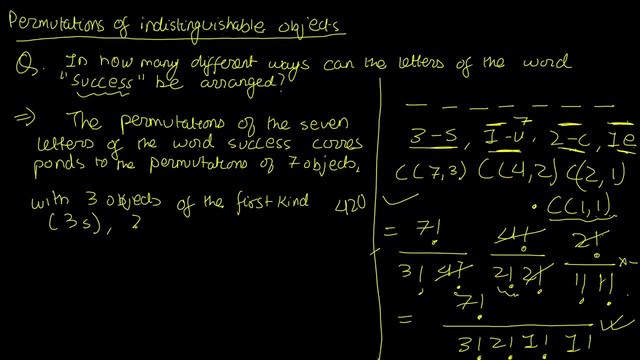 objects, with three objects of the first kind, two objects of the second kind and one object each for the third and fourth kind. This is given by- and we can apply this formula: is given by seven factorial, by three factorial times two factorial, And this is equal to 420.. Now, if you like, 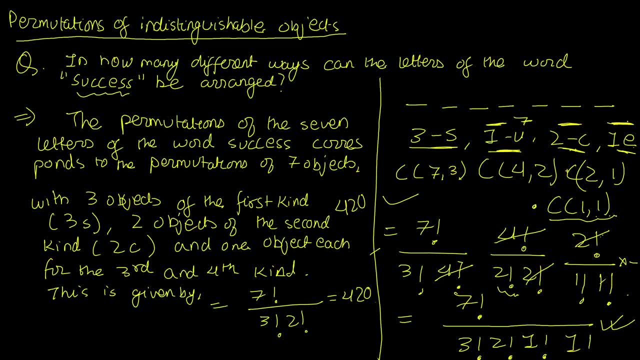 product of combination solution better. it would be completely correct to go that route. So just support your answer with the right arguments. For example, selecting three out of all seven positions for s, that leaves four different positions. And out of those four positions, 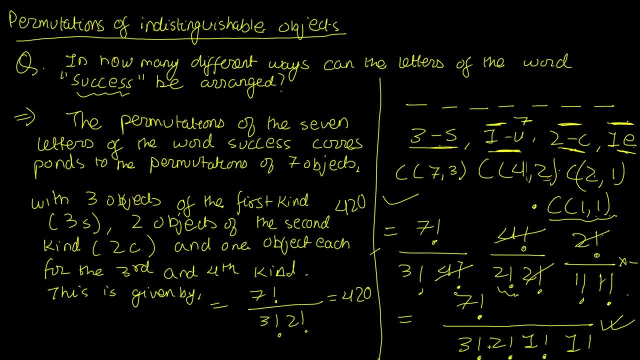 selecting two for c, And if you proceed that way, you'll get to the same solution. So, whichever solution you choose, just make sure that you express your ideas properly. Next, let's have a look at one more problem that generalizes this concept even further: How many ways are there to? 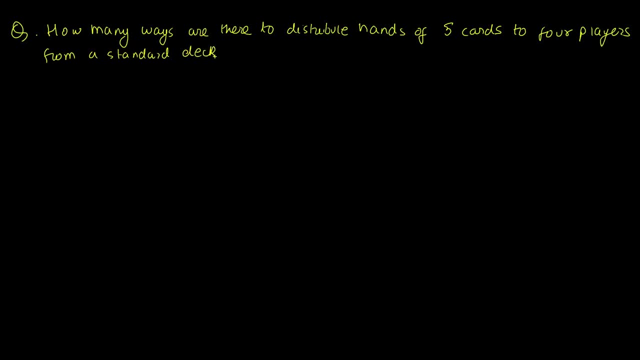 solve this problem. Well, let's say we have a total of 52 cards to four players from the standard deck of 52 cards, So the solution to this problem will also be pretty analogous to the last solution. I have a total of 52 different cards to start with. Now the first out of these four players. 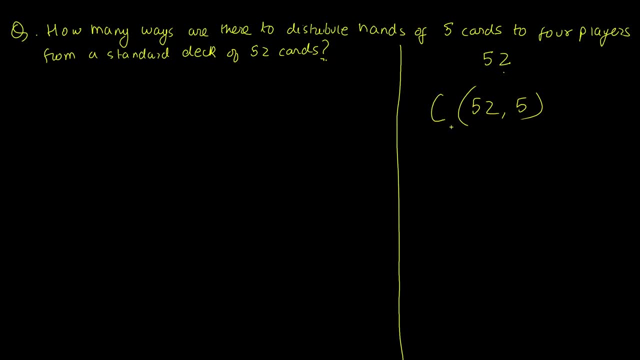 receives five of these cards. So I'll consider any random combination of five cards. And the reason I'm considering a combination is because when you're dealing cards, we're not considering the order in which the cards are dealt. This is because three cards are not on the same deck of the card, So there are only 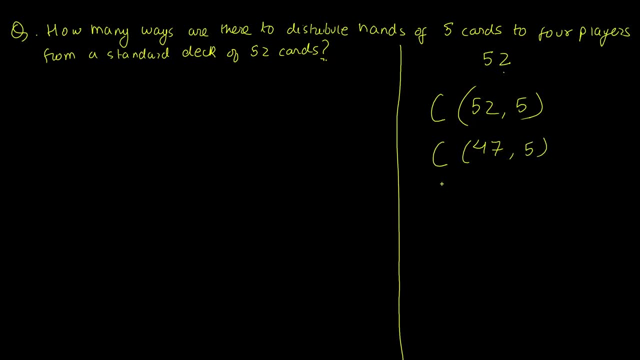 two cards to choose. There's only one card to choose, So the first card can only be a card for the second player And then for the third player it would be 42 comma five, and with 15 cards gone, the fourth player must be dealt from the remaining 37 cards. And so, if I take 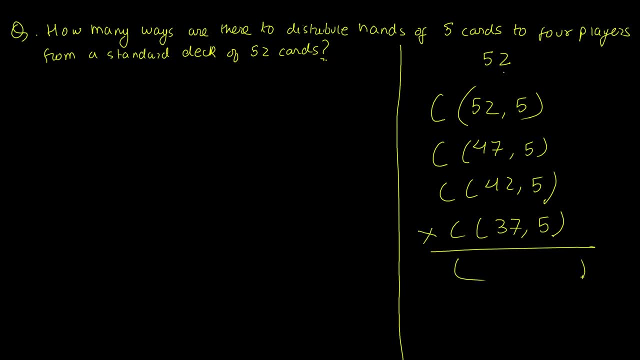 the product of these four combinations, I will get the answer that I'm looking for, But, believe it or not, it is exactly similar to the success problem we did earlier. But this word: we argued that there are a total of seven letters Out of the seven we 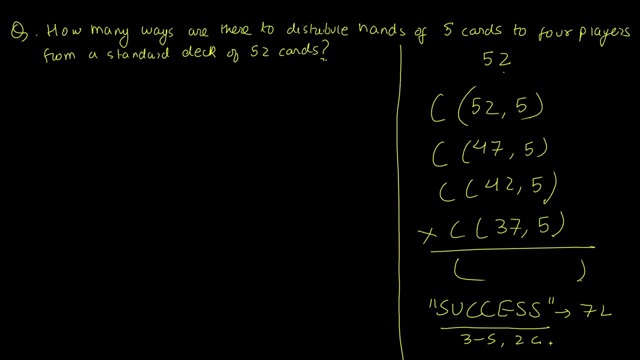 we had three occurrence of S, two Cs, a single U and a single E. And why is this? similar to dealing 52 cards to four players. You see, we can consider these 52 cards as the letters of this word success. So just like there are seven letters in this word, there are 52 cards. 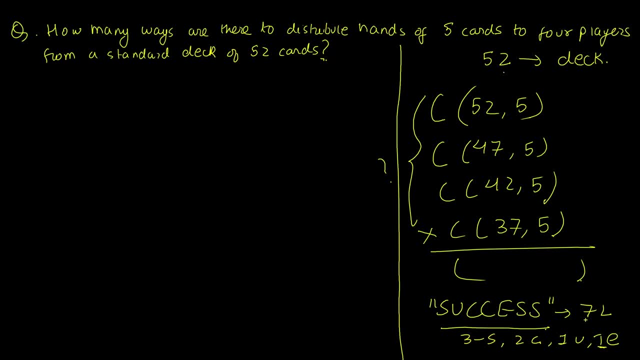 in this deck. And then we started making the groups Out of the seven letters we said there are three S, two C, one U and one E. Now, in our case, the 52 cards are divided in terms of the players and the deck. We know that after the dealing completes, there will 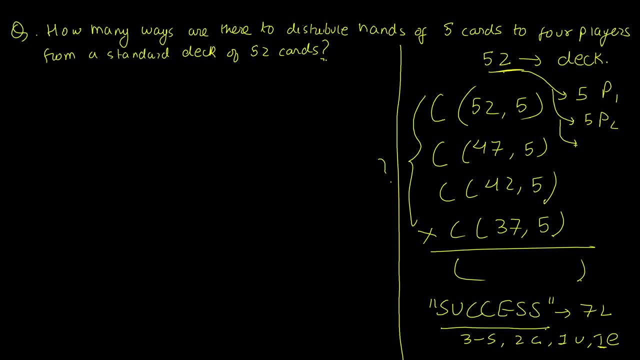 be five cards for player one, five cards for player two, five cards for player three and similarly five cards for player four. But is that all? No, this only accounts for 20 cards. I'll have 32 different cards left on the deck. So exactly in the way three S two. 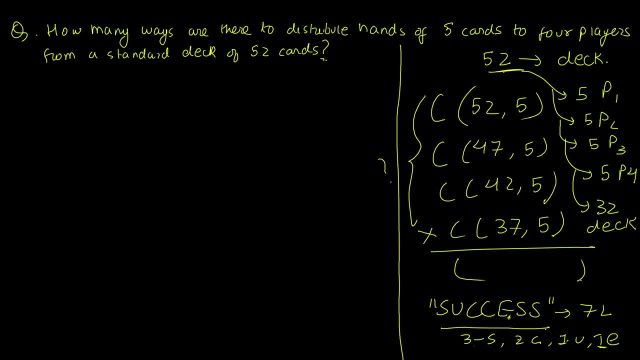 C, one U and one E is making of this word success. these four player distributions and the 32 cards distributed to the deck is the total number of cards that we have. So if I want to be technically precise, I'll need one more combination term in my product. 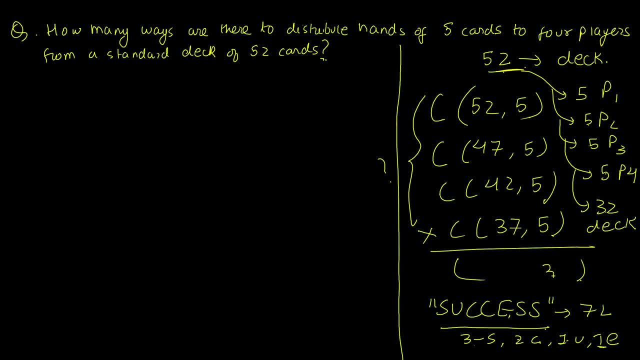 After dealing 5 cards to each player, 32 cards will go to the deck, But the remaining number of cards is also 32, so my final combination will just be C 32 comma 32.. And we know this is equal to 1.. So earlier I suggested that the product of these four combinations is: 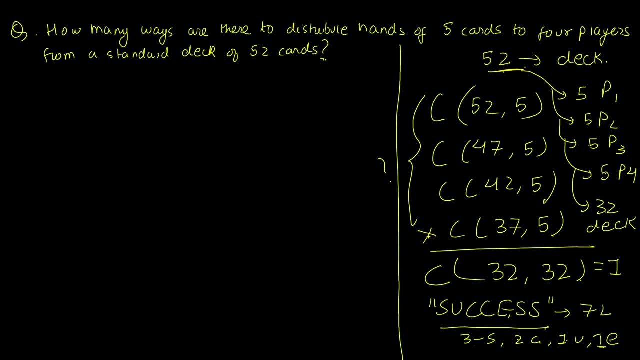 gonna be my result. That is technically correct. But we also need to understand that the last combination term is the result of the combination of all four. So we know that C will be the result of the combination of these four card. So if the result of the combination of these 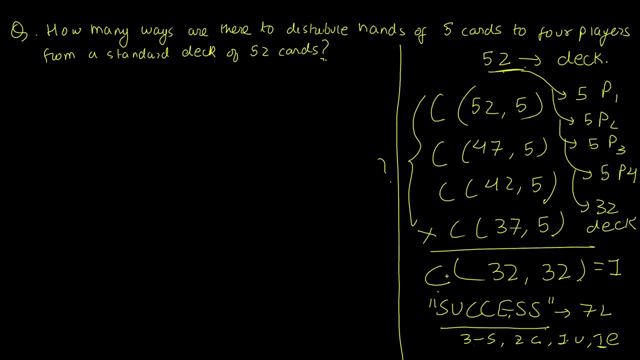 which is equal to 1, also appears in this product. so, looking into the approaches to solve this problem, if i just consider the product of combinations, i do not need to care about this number 32, but if i decide to use the repeated objects formula that i used in the success example, 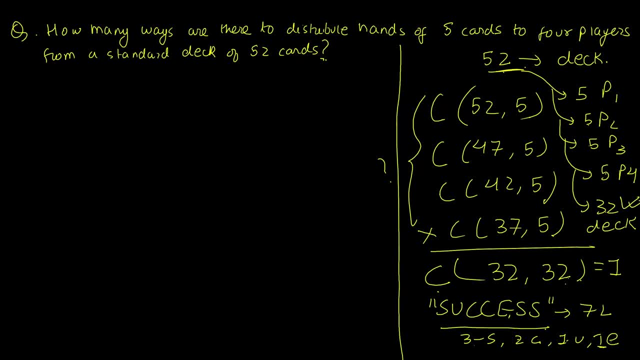 this remaining 32 cards in the deck- is important to consider, so this point will be even more clear. so let's proceed to the solution. so i'll use the approach of taking product of combinations. so i can start by mentioning the first: player is dealt 5 out of 52 cards and this has the 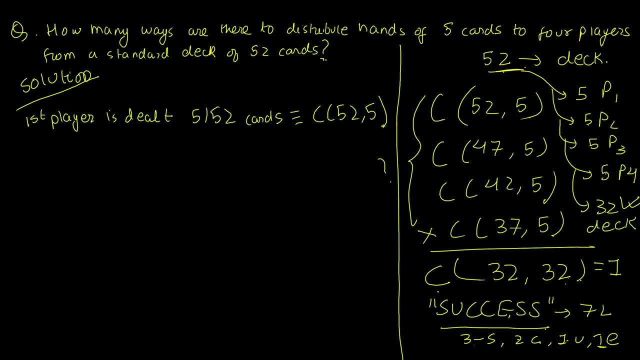 combination of 52 comma 5 possibilities. similarly, i'll list the other three players. i'll do that quickly and lastly, i want to mention that 32 cards remain in the deck, so you could think the remainder of the deck as being one more player that receives the 32 cards, and this one will just 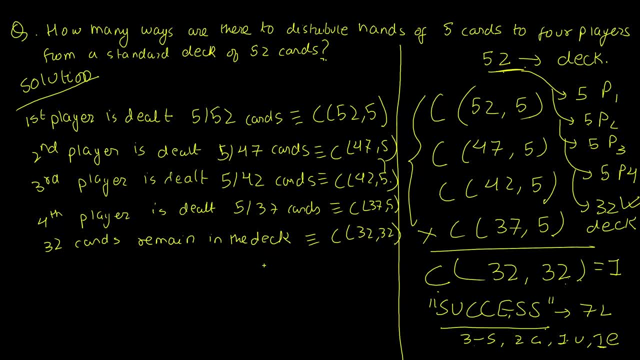 have the combination of 32 comma, 32 possibilities you. so to get to my result, we can simply apply the product rule. so my final answer is just going to be the product of these five combination terms and ultimately i can expand and cancel. but i can take the shortcut from this analogy. i know the result is going to be 52 factorial divided by the 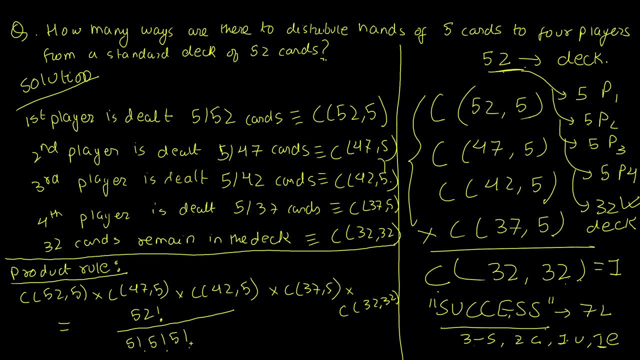 product of all these possibilities: 5 factorial 4 times followed by a 32 factorial so you can expand to verify that this combination product is the same as this expression, and this is typically how we leave this solution. so i'm going to take the shortcut from this expression and this is: 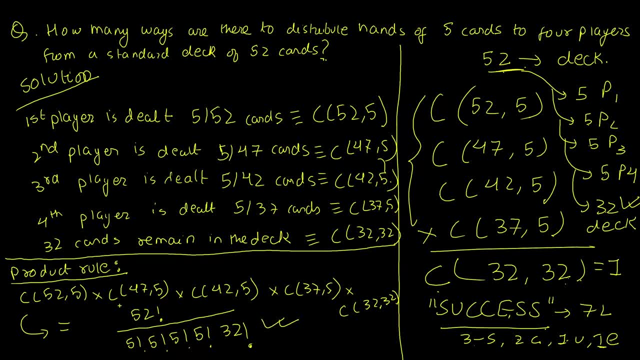 going to be 52 factorial divided by the product of those possibilities, and this is the solution. but the more important thing to know is that you could reach exactly this solution by following a different chain of argument, and that argument would be the same argument as you did in the. 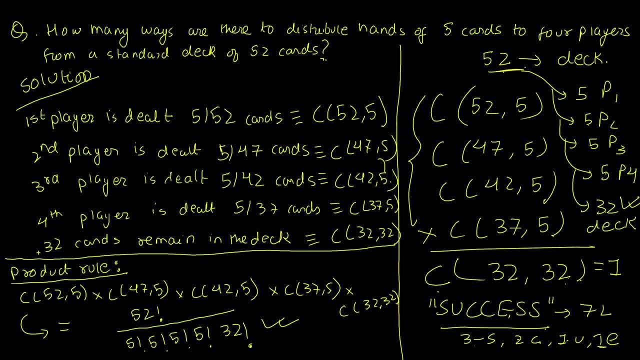 success example. so instead of arguing in this way about dealing cards, we could just argue that the problem is equivalent to finding the permutations of 52 cards, where five cards are of the first kind as in belonging to the first person, five more cards are of the second kind. five more cards are: 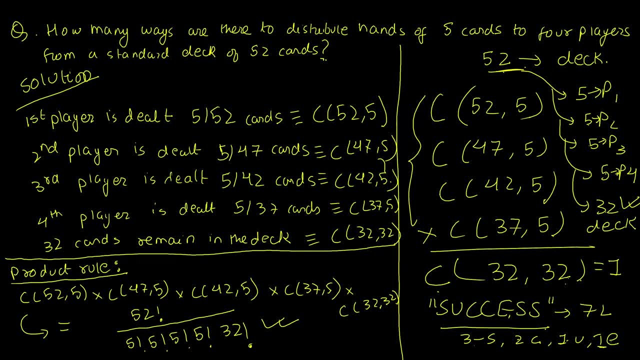 of the third kind. similarly, for the fourth kind, you can also find the permutations of 52 cards and and 32 different cards. for the fifth kind, that would be the deck, and you know that in that case this formula would also give the same result. and the most important thing to understand here: 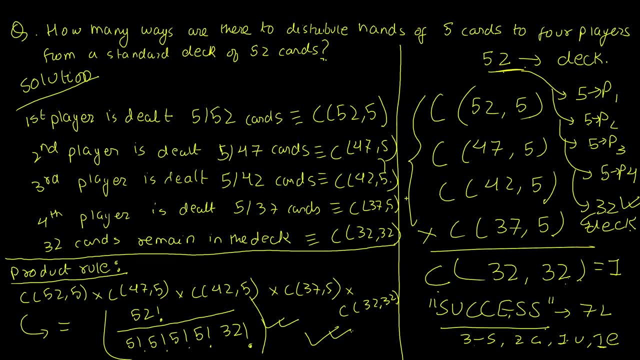 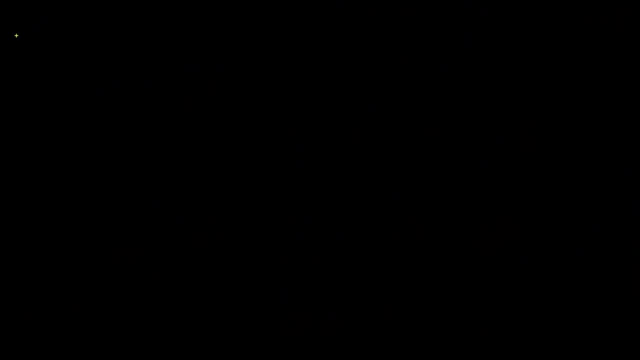 is that this formula is ultimately derived by taking this product of combinations. so this would be the more fundamental concept to understand. okay, getting on to the next problem: how many ways are there to place 10 indistinguishable balls into 8 distinguishable bins? okay, so whenever we see this kind of problem that involves indistinguishable objects placed in, 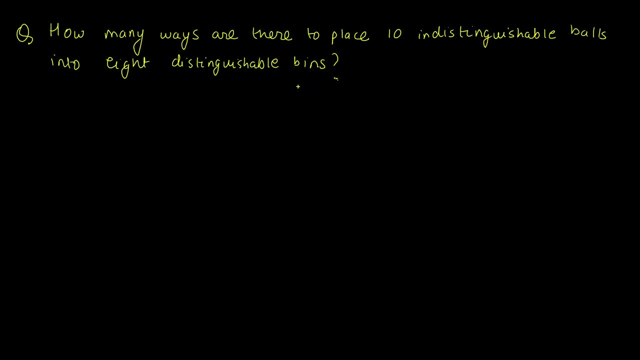 distinguishable bins or distinguishable boxes. we want to be able to relate to and borrow the concepts from combination with repetition. if we had a total of n categories and we looked at categories of fruits, apples, oranges and mangoes, so this would make three categories and we want 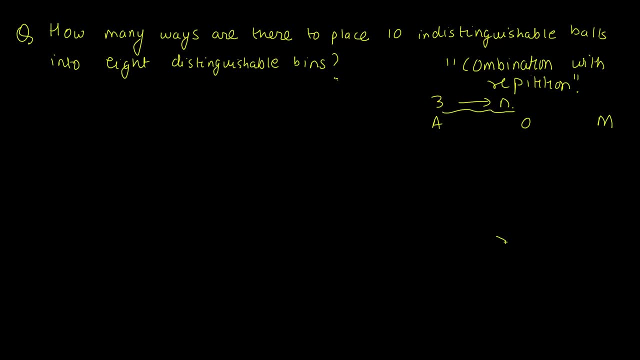 to generalize for n and out of these n categories i am selecting r items. please go back and watch the combination with me, with repetition and especially the main idea with dividers and stars, because, if you recall this properly, the way we solve this problem was by considering two dividers: one. 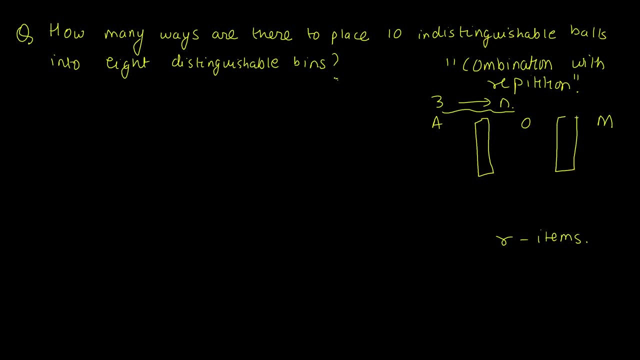 between apple and oranges and another divider between orange and mango, and we argued that for three categories we have two dividers. for n categories we would have n minus 1 dividers in general. and now, in order to select our items, all i wanted to do was to place our stars for 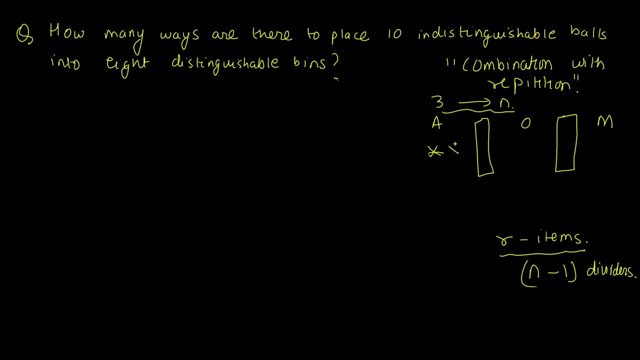 example, if i wanted to select 5 fruits, do so by selecting three apples, one orange and a mango, and therefore the number of these stars would be equal to the value of r and the number of the dividers would be one less than n- the number of choices. therefore, we came up with the final formula for combination. 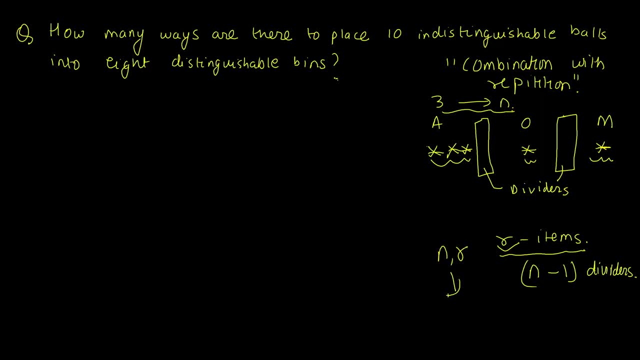 with repetition. for n objects taken r at a time. we say it would be the sum of stars plus dividers, n plus r minus one, taken with a combination against r. or this would also be equal to say n plus r minus one comma, n minus one, which is the number of dividers. 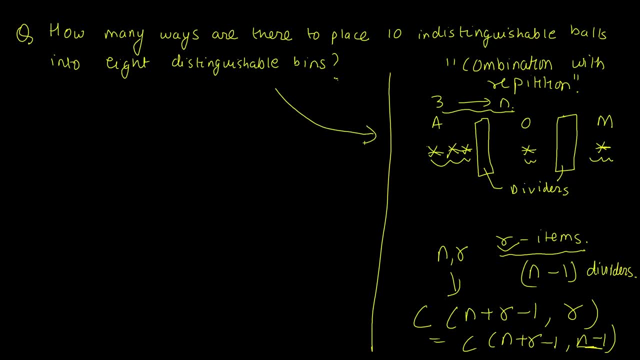 so now my job is to show you that this problem is the same as this one. first, I want you to agree that placing five fruits is the same problem as removing five fruits. so in this example we say: remove or select five fruits. when we looked at the problem of selecting, 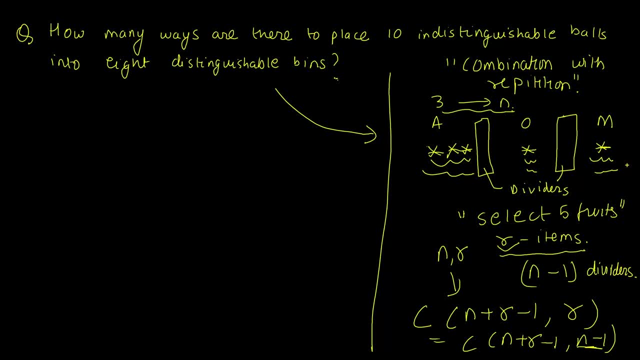 five fruits. we assume that the fruits are already in their respective sections, but that process of selection is exactly the same as placing the item back. so taking out is the same as putting in. so if we start with five fruits in your hand in the first place, we can look into the various ways the fruits can be placed. 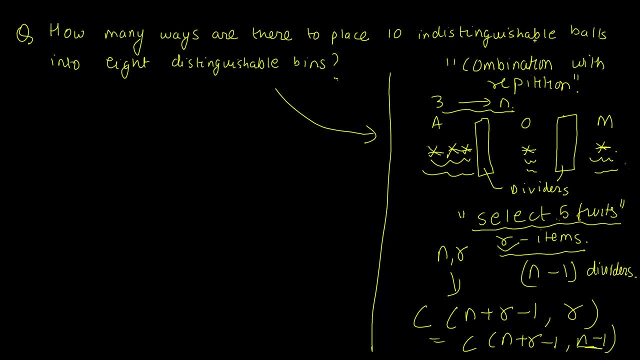 into their categories. now in this question it says that the balls are indistinguishable. that means one cannot be told to be different from another, but the analogy still holds in this case. I have eight distinguishable beans. I can still make eight different categories. 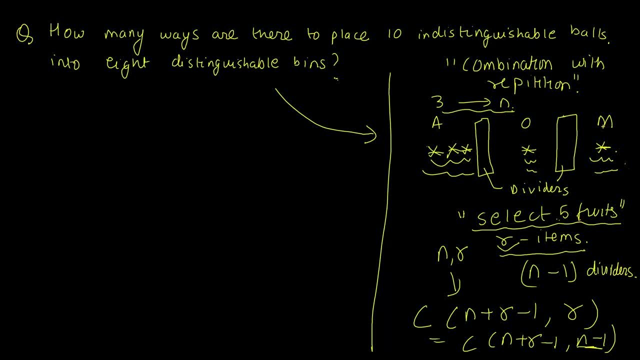 out of those beans, just like I did with my apple, orange and mango. so if I consider all the way up to eight different categories in my hand, then I can place in the second place and, as we did here, we are going to consider the seven different dividers between: 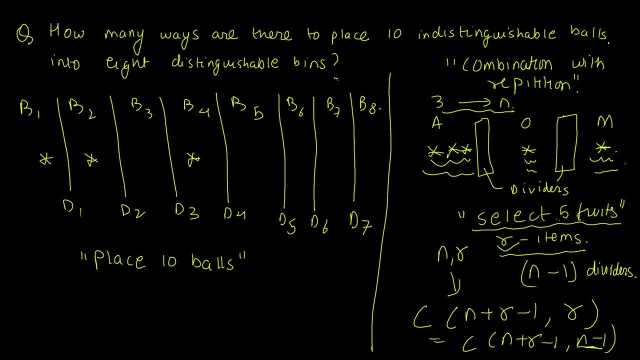 the eight beans. and now my job is to place ten different balls, and let me show you a random positioning of ten different balls by placing ten stars. so may be one here, two here, I'll take two of these. may be two of these, may be three of these and one of. 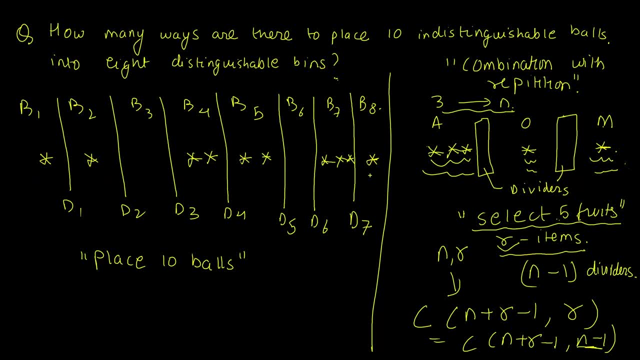 that. So by placing these ten stars in different ways, I can represent all the different ways: 10 balls into these bins and i know that each of my placement is analogous to the placement of these 10 stars and the 7 dividers. so 10 stars plus 7 dividers is a total of 17 different things. 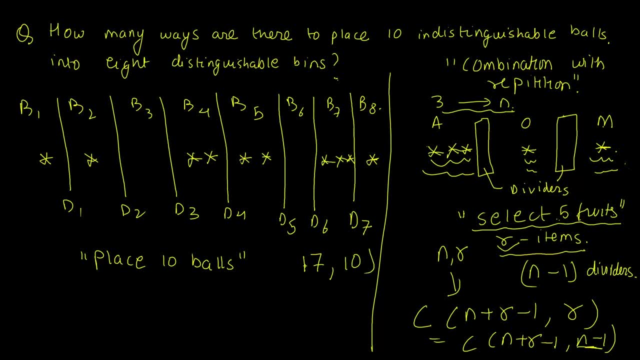 and in these 17 positions i either have to place 10 stars- see 17 comma 10- or i have to place 7 dividers- see 17 comma 7. these two will be equal and will be equal to my answer. so what is the? 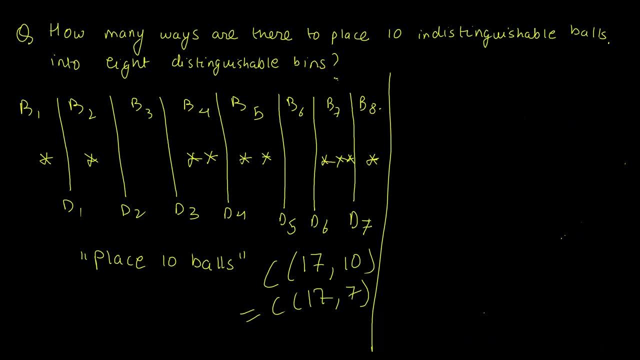 argument here. so i'll mention the formal way of answering this. in the right, the number of ways corresponds to the combination from a set of eight different objects, and these are my distinguishable bins. when 10 items are selected with repetition- and i hope you can see that analogy here we have. 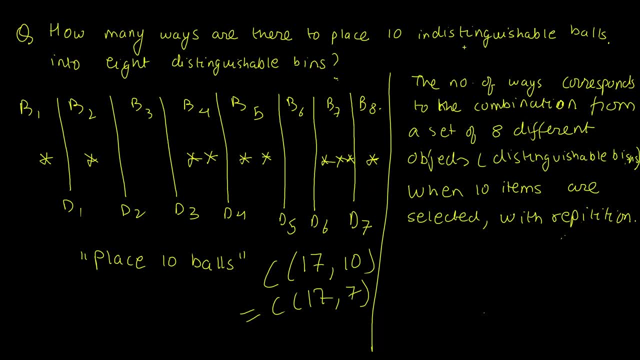 eight different bins representing my eight categories, and placing the 10 balls is same as selecting 10 balls and, with repetition, suggest that i could place or take more than one ball from a given bin, and we know that this is given by. this will be the combination of n plus r minus 1 comma r. 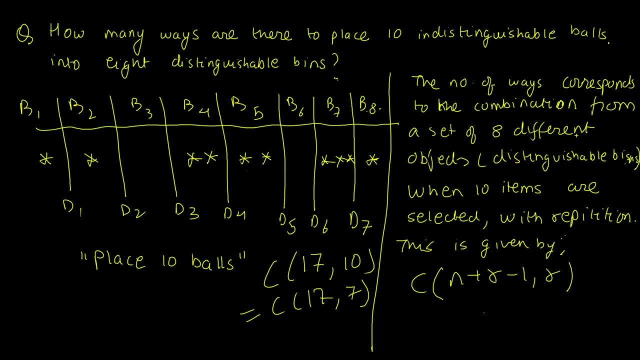 so the total number of categories, this 8 is going to be my n, the 8 different objects represents my n and the 10 items represents my r. so i'm looking for the combination of 17, because 10 plus 8 minus 1 comma and the second value is just going to be r, that is, 10 and this, as we talked about earlier. 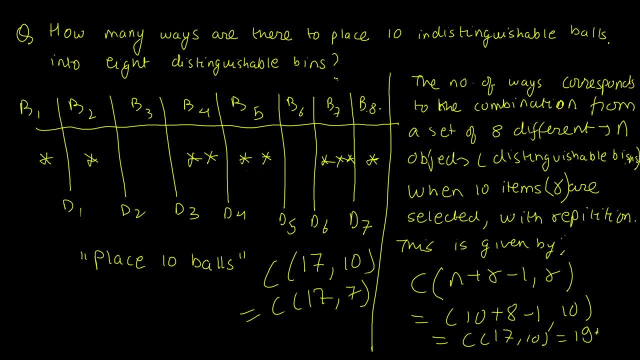 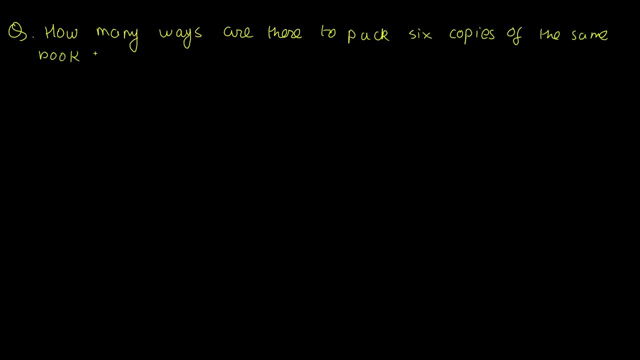 just see 17, comma 10, and this is equal to 19 048. okay, so we'll do one more problem: how many ways are there to pack six copies of the same book into four identical boxes, where a box can contain as many as six books? so this is a very deceiving problem. 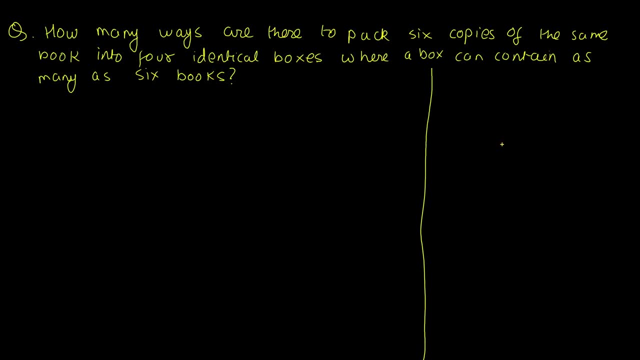 because it looks exactly the same as before, but it is not. when we looked into the last problem of 10 indistinguishable balls and eight distinguishable beans, these beans were distinct or different from each other when we considered our dividers and stars. so let's say i had three. 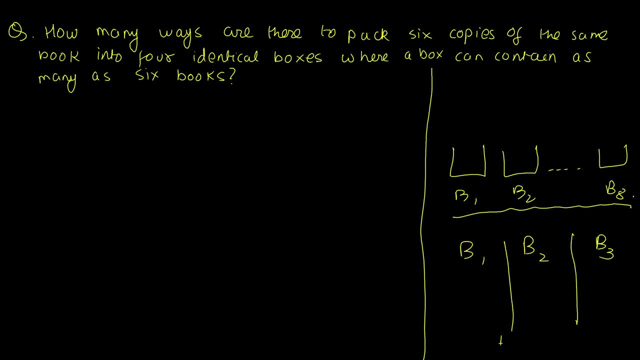 bins b1, b2 and b3. i would start by placing two dividers and i would place stars for my choices, and this choice of five would be considered different from this choice of five. and this one and this one are different because the number in the bin one, for example, is different. 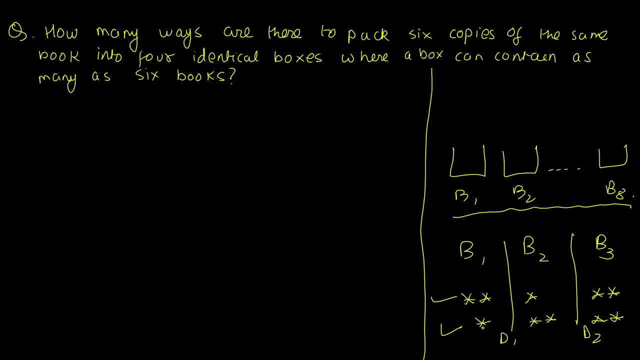 being one, only had two stars in this case, but in this case it has one. but in this problem the boxes are identical, The bins are identical, So bin 1 is the same as bin 2.. So I cannot really count these as two different permutations, Because if these two bins are the same, this configuration. 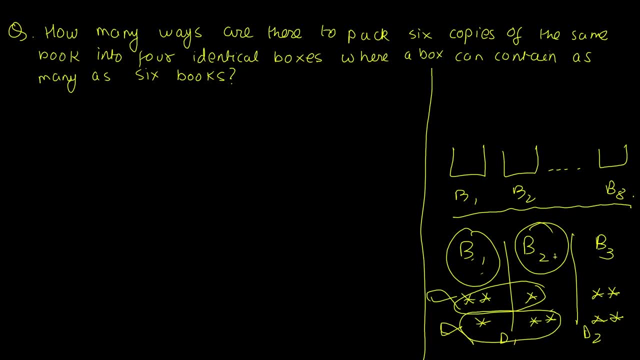 is exactly the same as this configuration In two identical bins. one has one star and the other has two stars. So our entire logic and the formula n plus r minus 1 comma r that we looked at earlier does not work in this situation. So when you see a problem like this, you have to be able to. 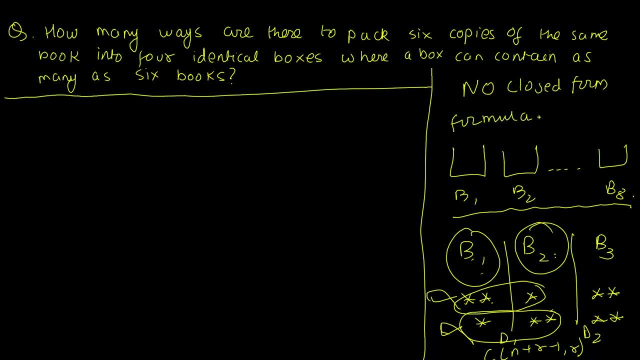 recognize it and there is no closed form formula, So we'll mention our answer this way. This problem involves indistinguishable objects and indistinguishable boxes. Therefore, we'll list all of the ways to pack the books. Each listing will be a sequence with a decreasing number of 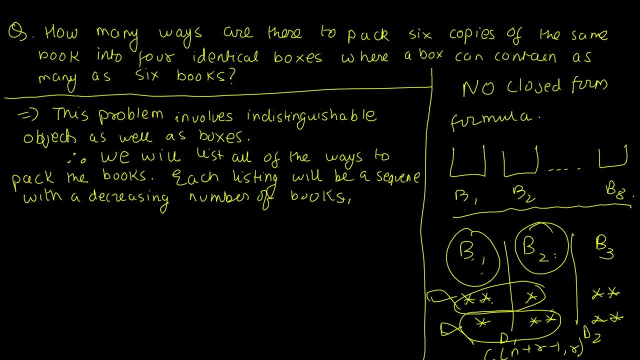 books. Okay, so in this case I have four identical boxes, So I do not want to specify distinct names and orders, But I know I need to pack six copies of the book, And so I'll mention that one of the possibilities is six. 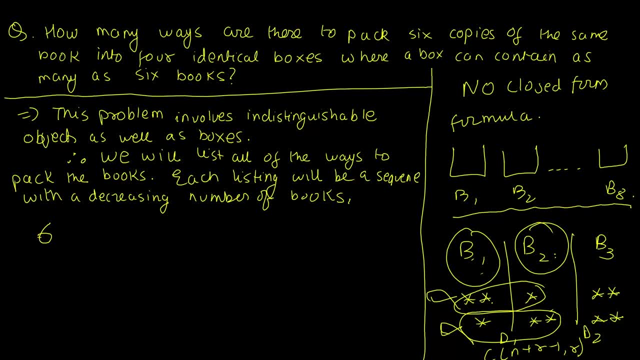 And this simply means that place six on any box and leave other three boxes empty. Okay, so I need to pack six books And I'm choosing to place all of them in one box, because a box can contain as much as six books, So I can choose to place all six in one box and the remaining are just zero. 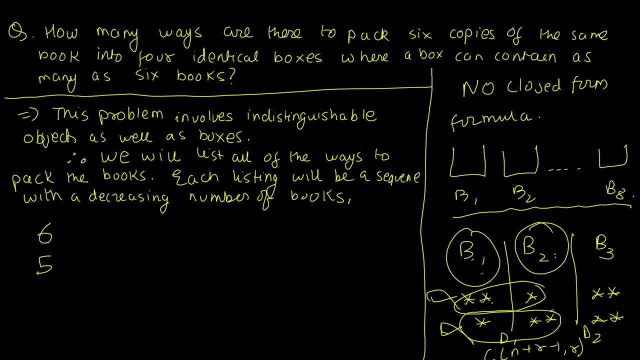 Another choice I could make is to place five in the first box, one in the second box and leave two other boxes alone. So I'll just mention the possibilities carefully, while making sure not to leave anything. So if I leave four on the first one, I could leave two on the second one, But with 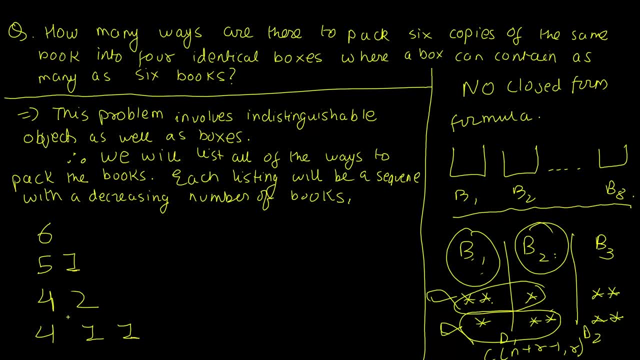 four on the first one, I could also do one, one, And I think that's all for four. If I have three on the very first spot, I could have three. on the second spot I could have three, two, one I could. 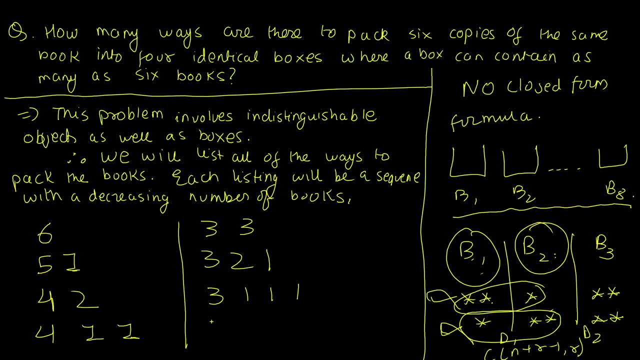 have three, followed by one, one, one, And that's all for three. I could have two, two, two And there could be one more. It could be two, two, one and one. So these are pretty much all the boxes. 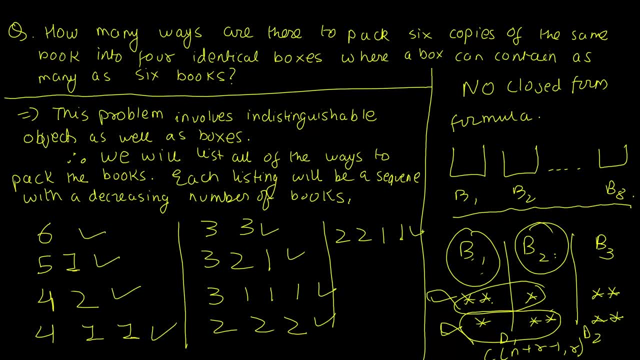 All the distinct ways in which you could place the books, And I hope you can see why this is happening: because the boxes are indistinguishable. I only need to say that put six in one box and leave three others alone. Leave three others empty. I do not need to specify which box to. 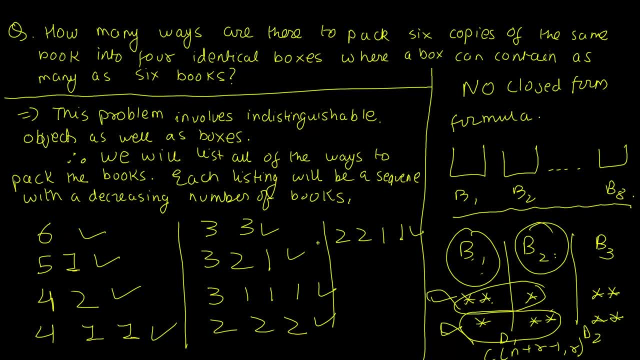 put the six ones in and which three to leave empty. In this case, I've used three boxes and left one empty. In this case, I've used two boxes, four on one, two on one, and left the order two empty. So the choice of the boxes that I'm making is completely up to you And I hope you enjoyed this. 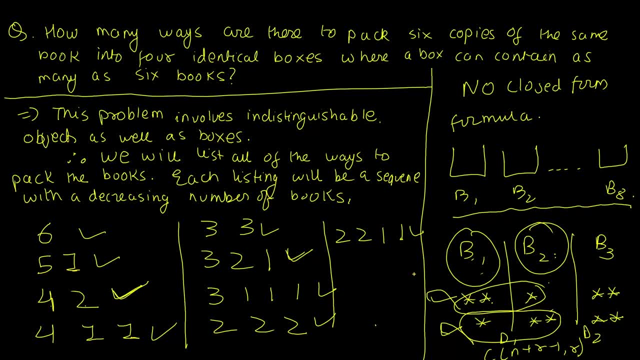 video. If you have any questions, please feel free to ask them in the comments. And if you have any questions, please feel free to ask them in the comments. But in this kind of problem, I hope you can see the difference. So from this point we'll just mention the very simple conclusion By: 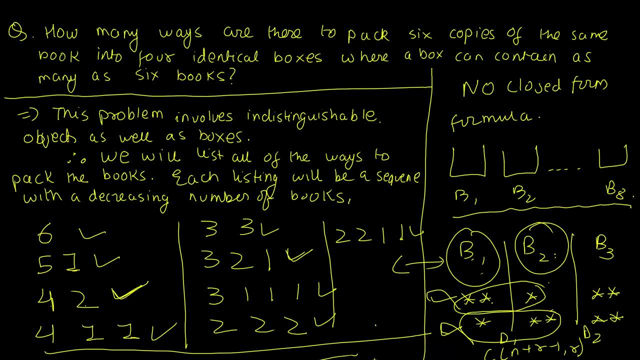 exhaustively counting, we can see that there are a total of nine different permutations or nine different possibilities. So with that problem we'll close the video for today. So we'll close this chapter in the next video with a look at the topic of generating permutations and combinations.